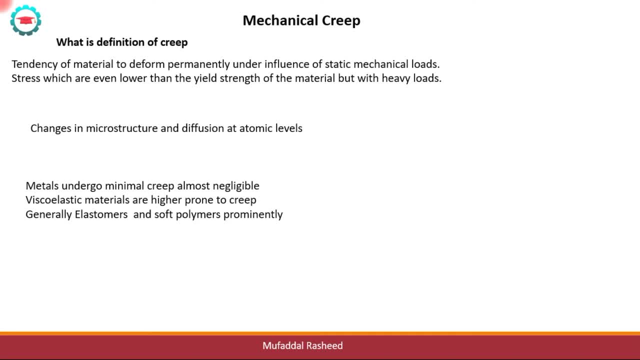 applications, except applications where there are very heavy loads which are involved. Visco elastic materials, on the other hand, are highly prone to creep. Examples being elastomers like rubber, polyurethane or soft polymers, They creep prominently. A good practical example of creep is the usage of rubber bushes in the mounting of shock observers. 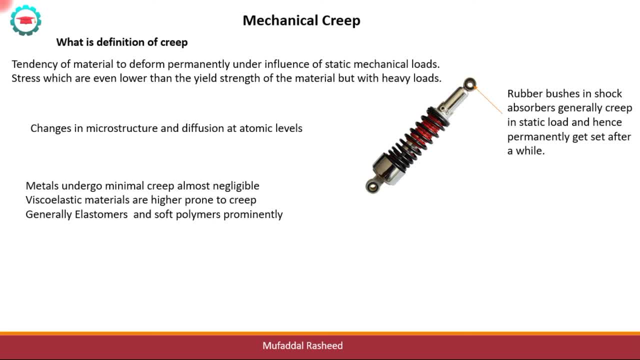 So shock observers are used in cars and bikes and they are mounted to the frame using rubber bushes, And these rubber bushes generally creep and they get permanently set after a while, after a certain amount of time for which the static load is acting. Another good example of creep is wood, So whenever wooden beams are used, 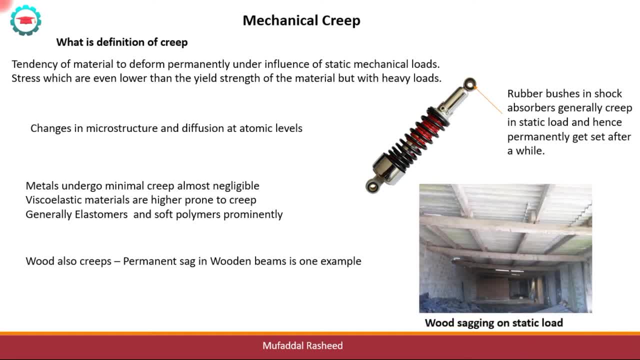 in structural housing type of applications, wooden beams generally sag, As you can see over here. these wooden beams are sagging Although the load which is acting on them might be well within the elastic limit of wood when it is being tested, but it will permanently sag. 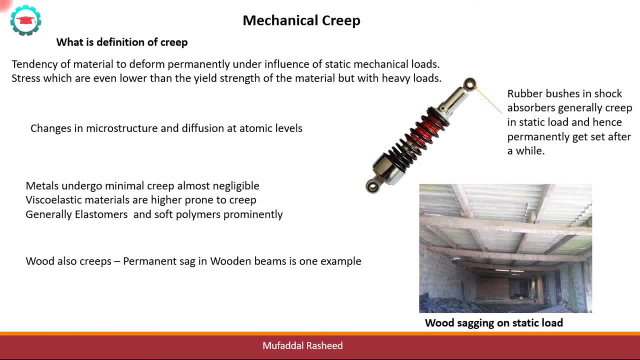 after a set amount of time. Creep, like other properties, is heavily dependent on geometry. So metals or steels generally don't creep much as compared to wood or elastomers. But when metals are used in the form of sheet panels- let's say the example of an automotive body- body sagging- 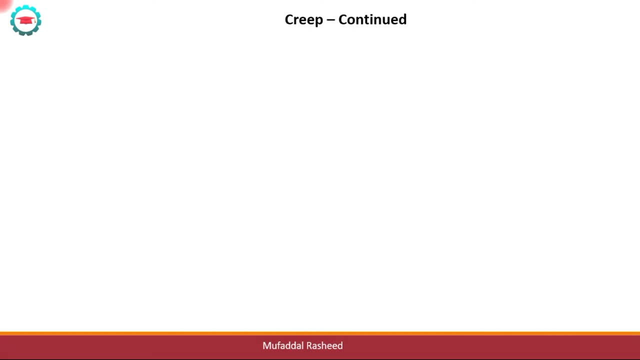 is one example of mechanical creep. So creep generally takes place in three stages, As you can see over here: primary, secondary and tertiary. In the y-axis it is strain, epsilon and x-axis it is time. So when the load is applied at t0, a static strain will take place. 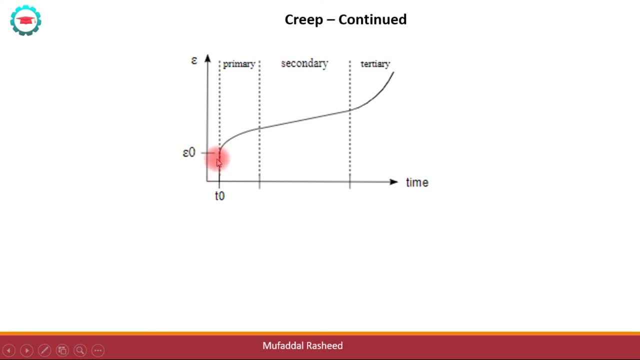 that is epsilon 0.. That is shown over here at t0.. Instantaneously there will be some amount of deformation, which is the static strain, And then, as time passes, the strain will gradually increase with respect to time, which is the primary phase. 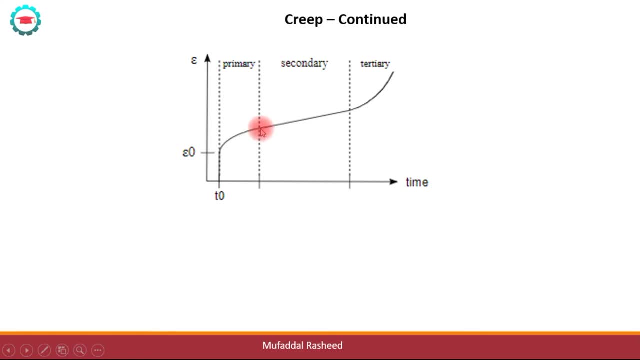 So it will start increasing at a steady rate. So this secondary phase is highly steady, which is shown over here as a straight line, And then finally, in the tertiary phase, the strain will increase much faster with respect to time. So this phase, that is, a secondary phase, is generally